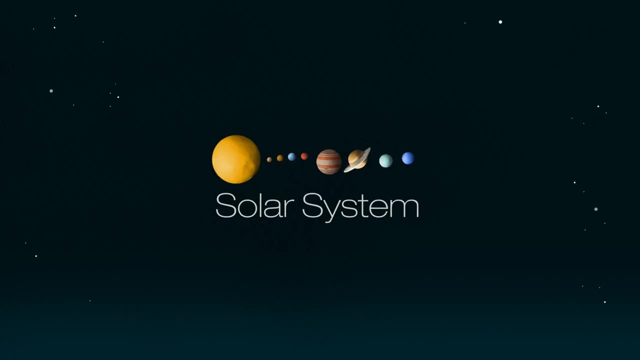 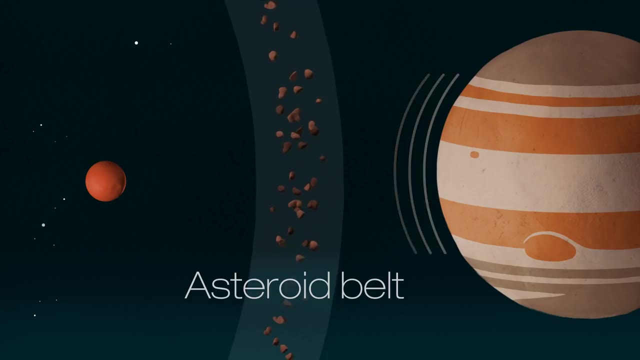 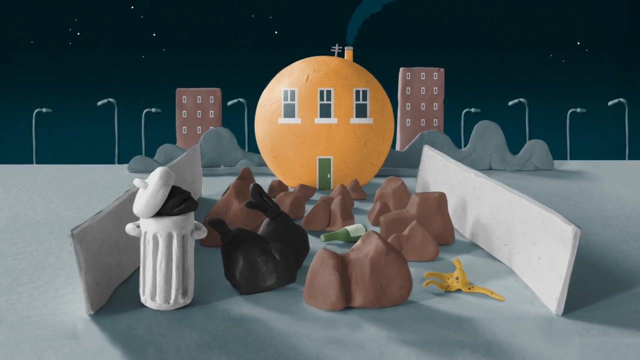 Space rocks. Our solar system is a vast and fascinating place. Between Mars and Jupiter we find the asteroid belt. Due to the mighty gravitational effects of Jupiter, these chunks of rock and metal couldn't come together to form a planet and instead made up a solar junkyard of sorts. 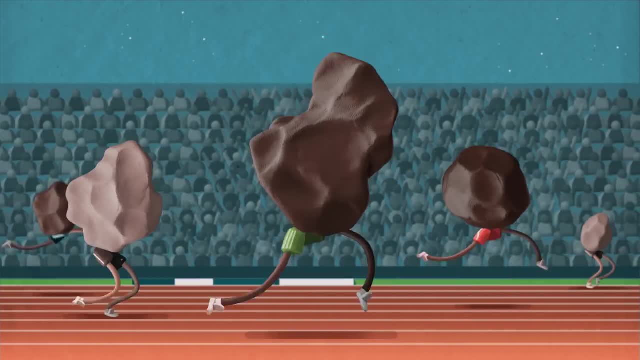 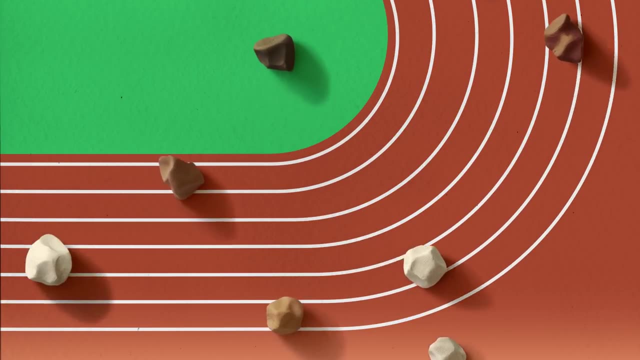 This is a crowded place to be an asteroid. Sometimes they collide with each other and get knocked off course and even out of the belt altogether, on a very different journey through the solar system. There are lots of names associated with space rocks, so what's the difference? 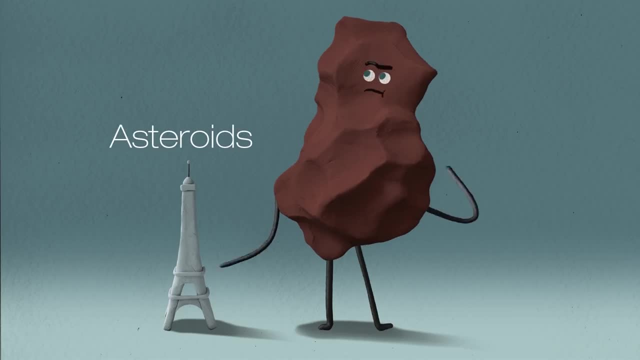 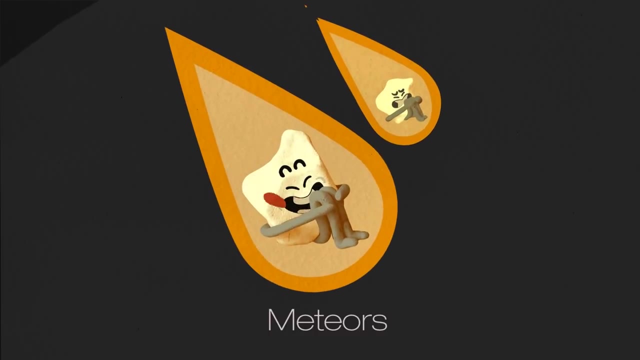 Well, the bigger rocks are called asteroids, The smaller are meteoroids, And when they fly through the Earth's atmosphere, they are called meteors. If they manage to survive their burning descent through our atmosphere and land on Earth, we call them meteorites. 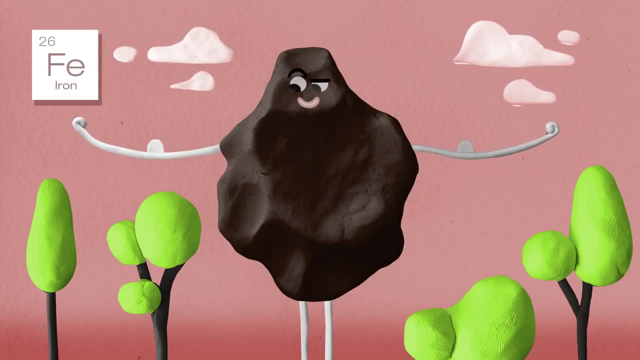 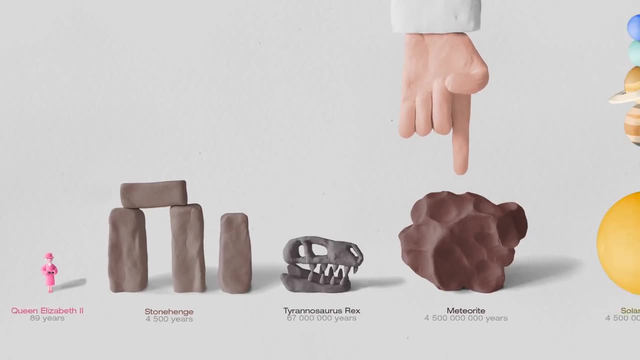 Some meteorites contain iron, which makes them very dense, dark and magnetic. They are the oldest thing you could ever touch, as they are the same age as us. That's the solar system. The gas giant, Jupiter, marks a boundary in the solar system called the snow line. 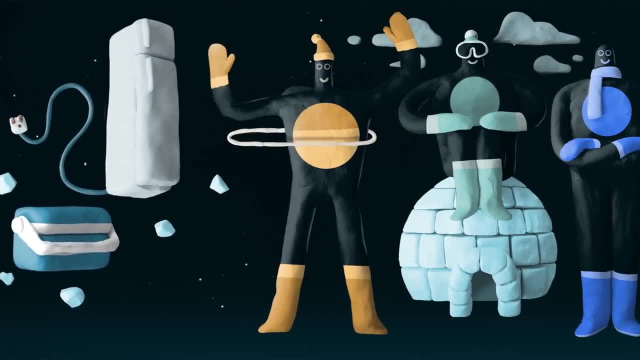 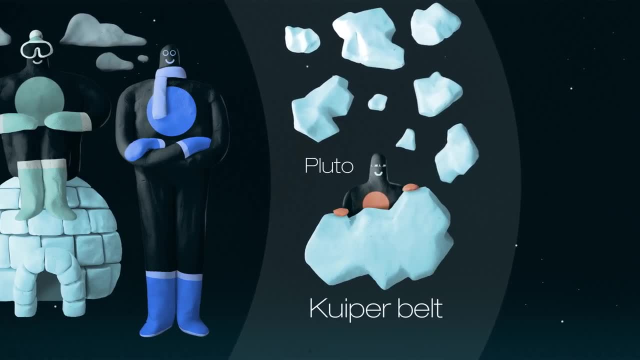 beyond which objects contain a lot of ice Past- the other three gas giants- we find a huge ring of ice chunks, large and small, called the Kuiper belt, where the dwarf planet Pluto lives. Even more of these ancient, dirty snowballs exist in a huge bubble called the Oort cloud. 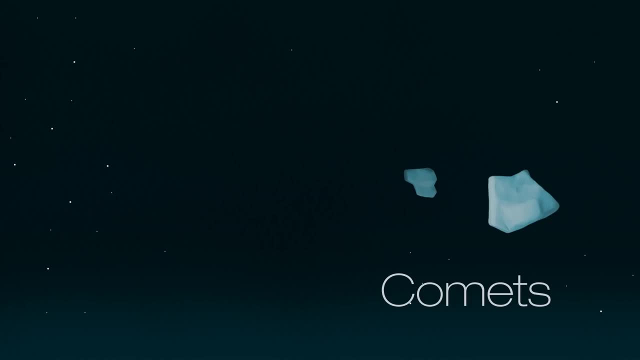 These icy objects can get bumped off course, sometimes to become comets that journey past the planets towards the Sun. Some collide with other objects and get smashed to bits. Others head towards the Sun and form long, beautiful tails as their icy surfaces warm up. 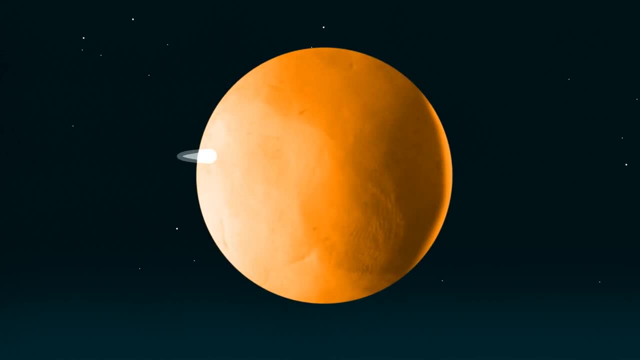 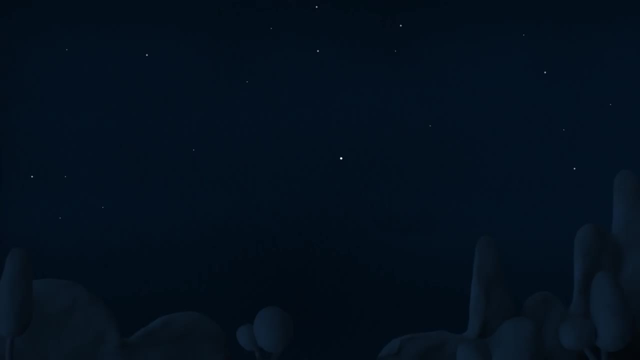 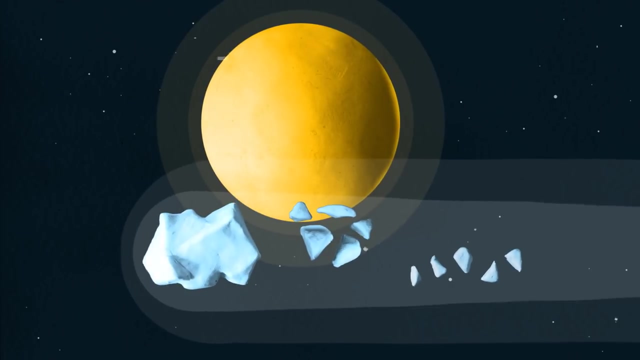 Here. they will either fall into the Sun never to be seen again, or they will survive and speed back home beyond the snow line. Here on Earth, we are treated to spectacular natural firework displays in the sky from orbiting comets. As they get close to the Sun, they burp, splutter and crumble, leaving behind a trail of debris. 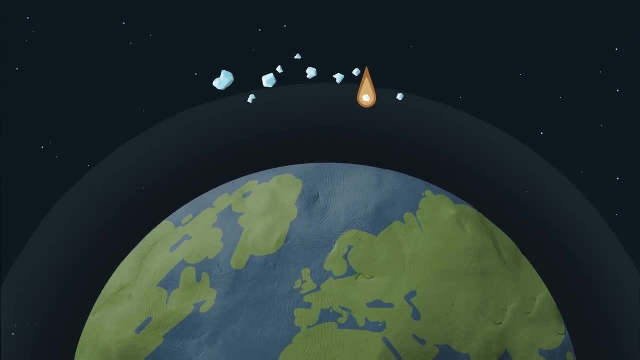 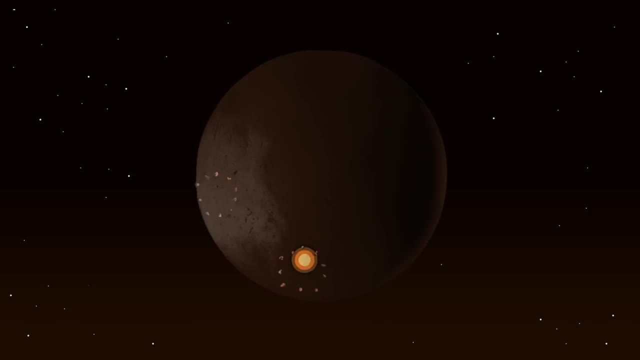 At certain times of the year, the Earth ploughs through these trails and bits of comet flare up as they fly through our sky and become comets. The early Earth was hit by thousands of comets and asteroids. It is thought they brought water to our world.